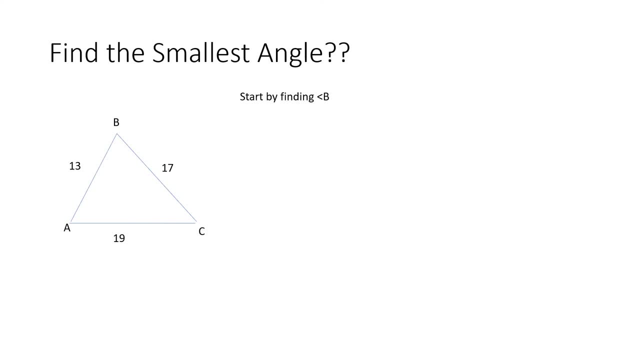 Ok, let's start by finding angle B. Formula B squared equals a squared plus c squared minus 2ac times the cos of b. Substitute the values that we have in our diagram into the equation, So 19 squared is equal to 17 squared plus 13 squared minus 2 times 17 times 13 times. 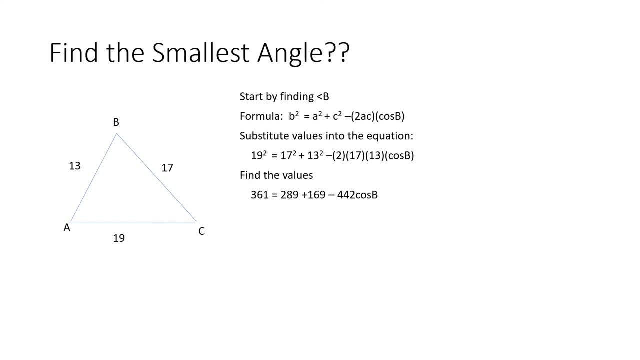 the cos of b. Now find the values: 19 squared is 361.. 17 squared is 289.. 13 squared is 161.. 269 minus 442. cos b. Move all the numbers to one side and the unknown value to the other. 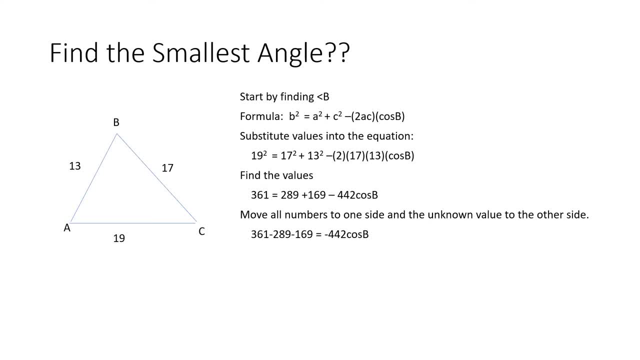 side, We will get 361 minus 289 minus 169 equals negative 442 cos b. That's simple. That simplifies to negative. 97 equals negative 442 cos b. Divide both sides by the number in front of the variable, which is negative 442.. So we will get negative 97 divided by 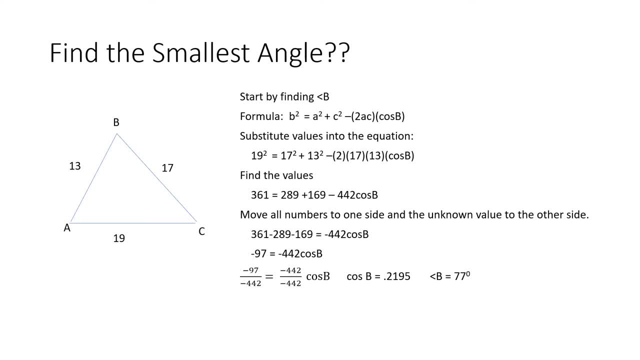 negative 442 equals negative 442 divided by negative 442.. Now we will get the angle B. YOUR Rgee is that opposite of that. So the angle B is 0.2195,. give 77 degrees at angle B. 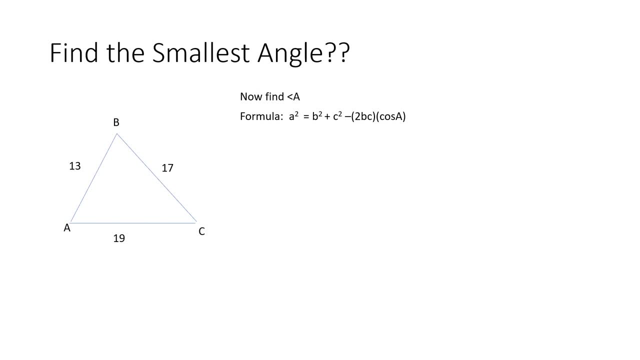 Now angle A. We re-write the formula: A squared is equal to b squared plus c squared minus 2bc times the cos of a. Our angle B coordinate art class minced gäller angle B. It's used when we want to multiply the angle B with the zero angle of the mu. 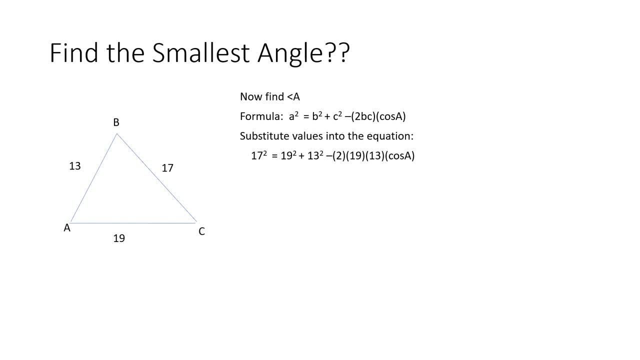 When you progress them into a givenatiques theorem, it requires a corresponding directive. That will give us 17 squared equal 19 squared plus 13 squared minus 2 times 19 times 13 times the cos of A. Now we'll do the calculations. 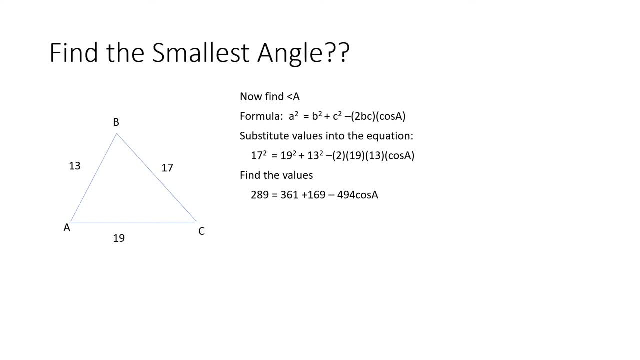 289 equal 361 plus 169 is negative 494 cos of A. Move all the numbers to one side and the unknown value to the other side, So we will get negative 241 equal negative 494 cos of A. Now divide both sides by negative 494.. 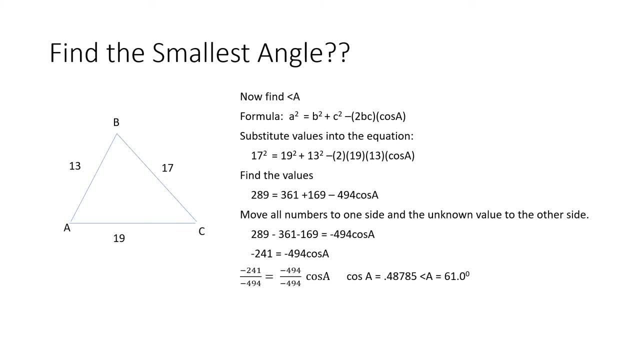 And you will then put that number into your calculator and get: the cos of A is 0.48785.. So angle A is 0.48785.. And you will then put that number into your calculator and get the cos of A. So angle A is 0.48785.. 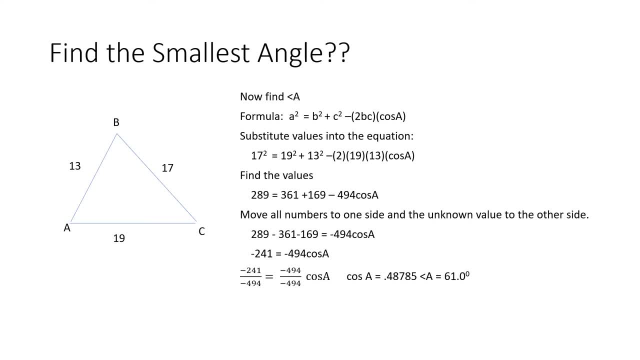 And you will then put that number into your calculator and get the cos of A. Now we will find angle C. We'll rewrite the formula: C squared equals A squared plus B squared minus 2BACOS of C. Substitute the values given in the question into the equation. 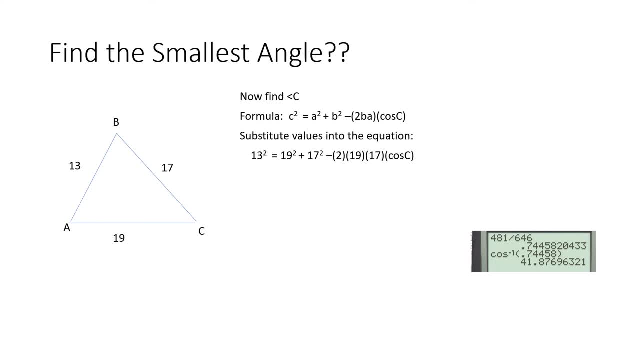 13 squared is 19 squared plus 17 squared minus 2, times 19, times 17,, times the cost of C. Find your values. So we get: 169 is equal to 361 plus 289, minus 646, times the cost of C. 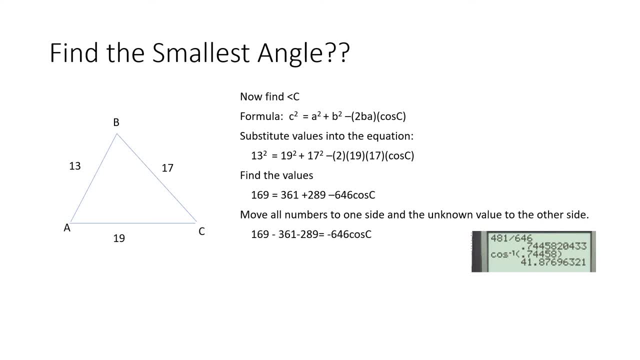 Move all the numbers to one side, the unknown to the other- We'll be getting really good at this by now- And then simplify. So we will get negative 481 equals negative 464. cost of C: Divide both sides by negative 646.. 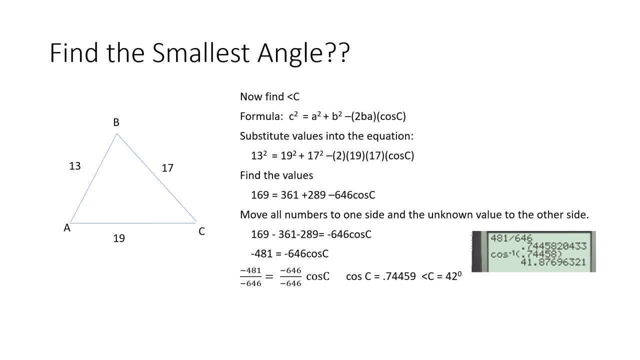 And you can see that will give me a decimal of 0.7445, which is the cost of C value. So angle C is 42 degrees. Conclusion: angle A is 61 degrees. angle B was 77 degrees. angle C is 42 degrees. 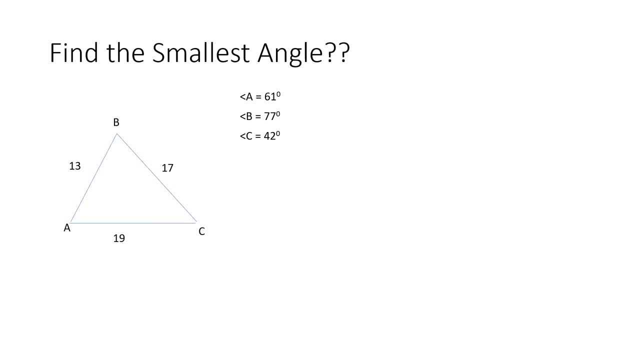 Now keep in mind how you labeled. your values might be slightly different, but the smallest angle is 42 degrees, which is 100% correct.